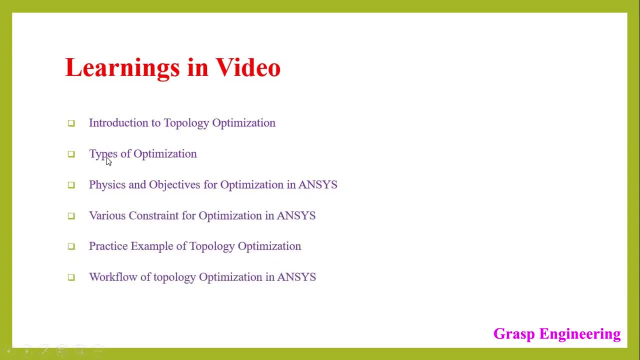 the topology simulation is a topology simulation, So this slide represents the learnings in this video. As discussed earlier, the topology simulation is a topology simulation, So this slide represents the learnings in this video. As discussed earlier, the we need to first see the small introduction, then we will going to see what are the major types of. 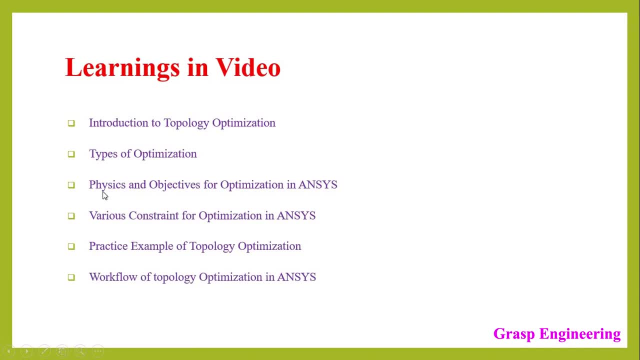 optimization, and then we will move to our ansys part. So, like there, we will see what are the physics and objectives when we used to talk about optimization in case of ansys. Then we will also discuss about what are the various constraints, like manufacturing constraints in case of 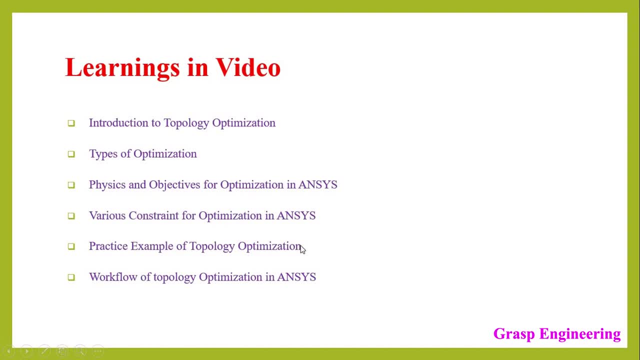 optimization, and then we will see the one of the practical example which is already done, and then we will discuss about the workflow when we talk about the optimization. So this slide represents the learnings in this video. As discussed earlier, the topology simulation is a topology simulation. 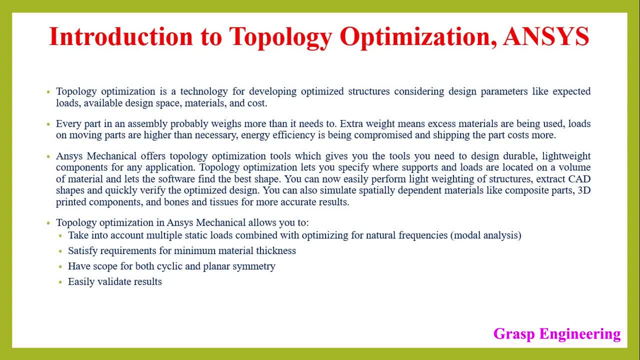 So this slide represents the small introduction to topology optimization. So topology optimization is a technology for developing optimized structure considering design parameters like expected loads, available design space, material and cost. So, in short, as name suggests, optimization is a process where we need to obtain the optimized 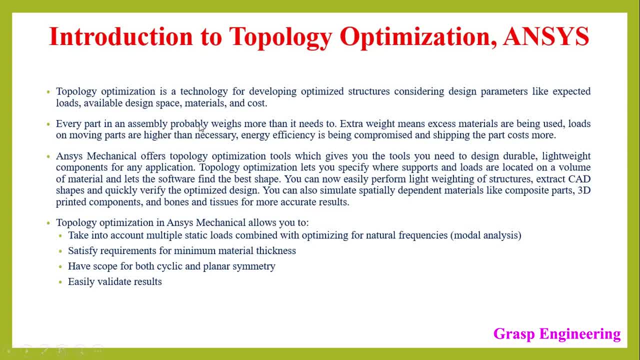 structure. So every part in assembly probably weights more than it needs to. So extra weight means excess material are being used, loads on a moving parts are higher than necessary, energy efficiency is being compromised and shipping the parts cost more. So, in short, that when we used to do overdrive, 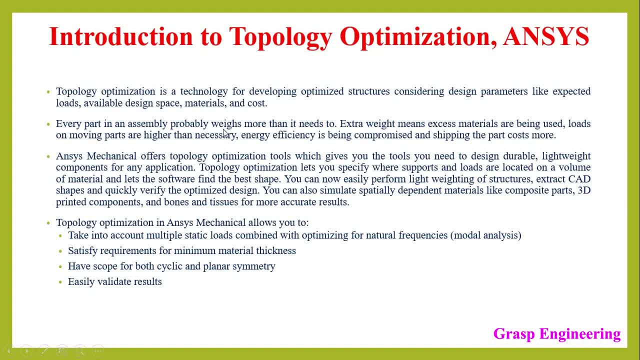 design of the structure. in that case it results into excess weight. So this excess weight may result into excess load on a moving parts and unnecessary it will affect the energy efficiency. It will also involves the shipping cost for the transportation. So all these results due to only 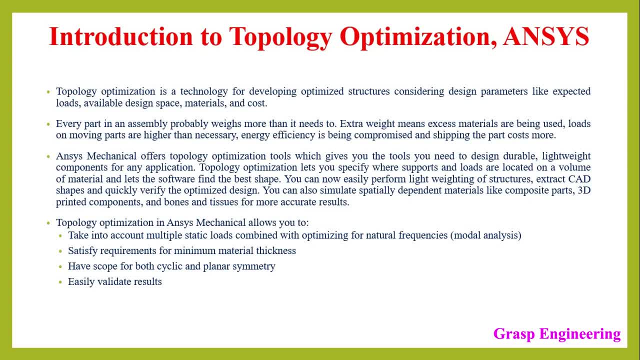 the excess weight. So for that case we need to think for this optimization. So nowadays most of the industries are using this optimization to optimize the parts. So now let's take a look at the optimization of the structure in design phase itself. so ansys mechanical offers topology optimization. 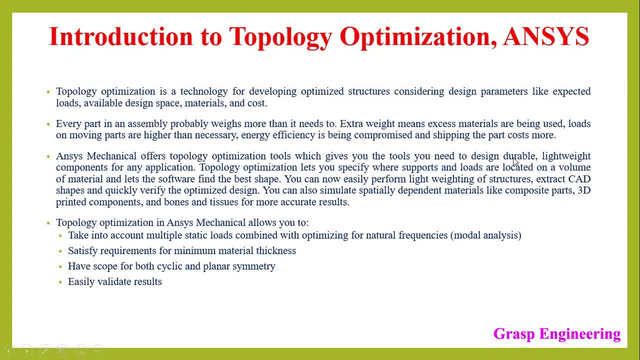 tools, which gives you durable design, light will component for any applications. so topology optimization lets you specify where the supports and loads are located on a volume of a material and lets this software finds the shape. so, basically, whatever the operational loads are there on structure, as well as what are the supports, that we can easily define and we can define that. 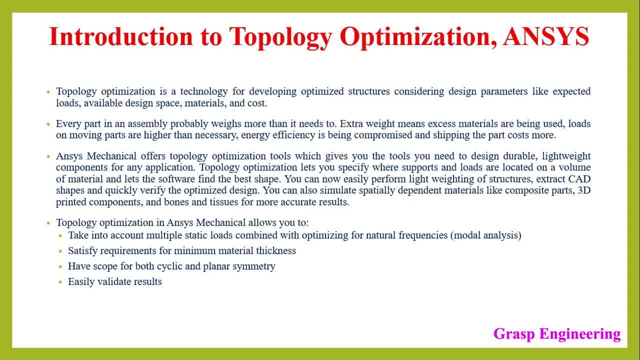 in a respective volumes, and then we can easily obtain the optimization with the help of ansys tools. so you can now easily perform light wing of a structure, extract CAD shapes and quickly verify the optimized design. you can also simulate particularly dependent materials like composite parts, 3d printed. 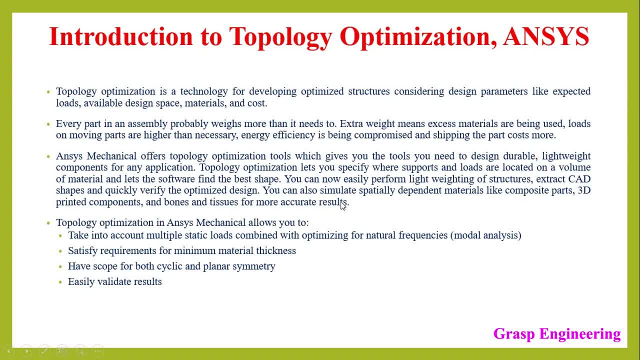 components, bones and tissues for a more accurate results. you can also simulate particularly dependent materials like composite parts, 3d printed components, bones and tissues for a more accurate results. so these are the major application, as we know that tissues and bones like when we talk about medicals application, so in that case this optimization nowadays are: 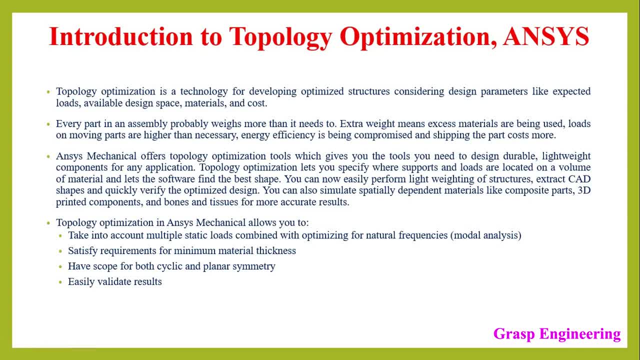 increasing, as well as 3d printed part. so this 3d printed part you can easily design with the help of this optimization tools. when we talk about ansys mechanicals, it allows us to take into the account multiple static loads combined with optimizing for a natural 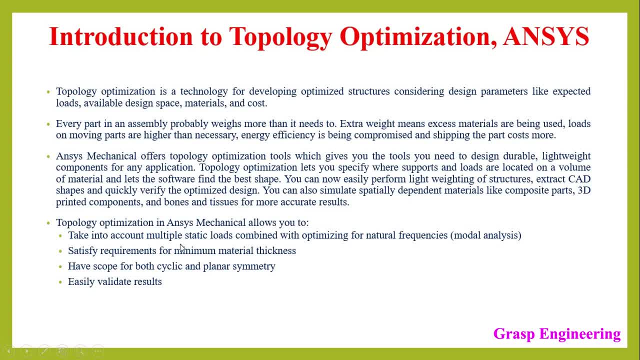 frequency. so, in short, that model analysis, along with the static loads, we can easily incorporate in case of topology optimizations. so it satisfied the requirement for minimal material thicknesses, have scope for both cyclic as well as planar symmetry, so we can easily perform cyclic as well as. 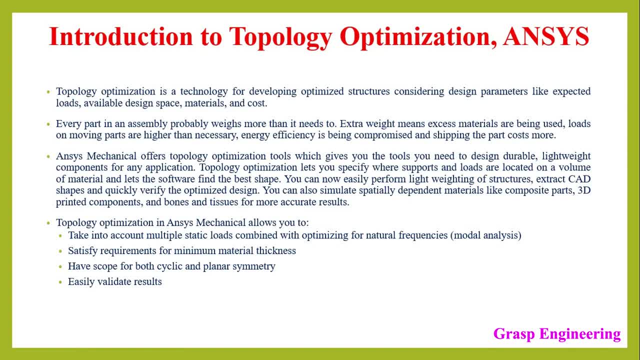 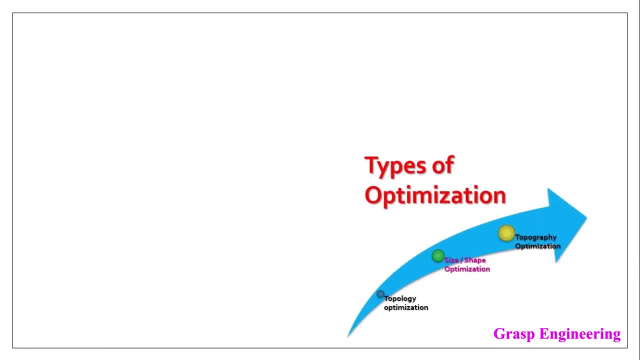 planar symmetry in case of topology optimization with the help of ansys, and also we can easily validate the results for the optimized structure. so in previous slide we discuss about the small introduction to optimization. now let's discuss about the. what are the major types of optimizations? so when we 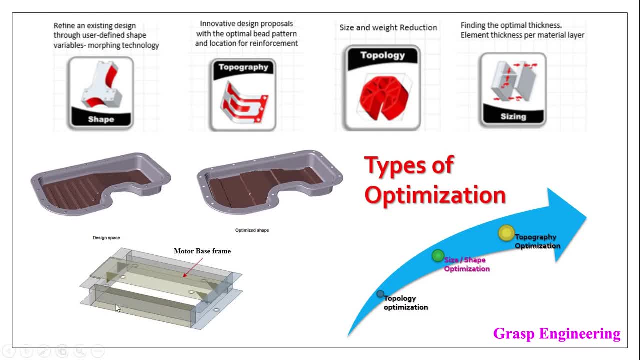 talk about optimization, there are four major types like. the very first is like topology optimization. the next one is your size, then makes the shape optimization and then next is topography optimizations. so when we talk about shape optimization, that then here refined and existing design through user-defined shape variable morphing technology. so here, basically, 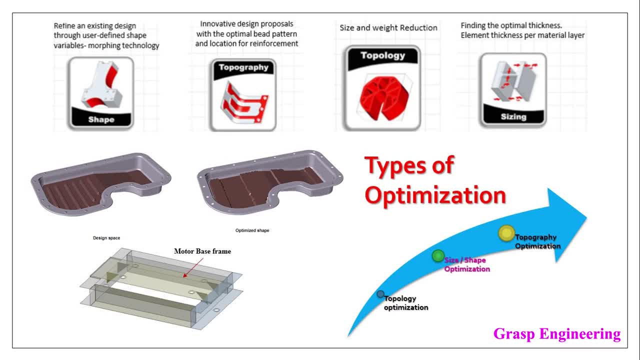 we used to use user-defined shapes like- just talk about this example. here we have some. first, initially, you have a rectangle, and then you define some shapes by putting this curves, as well as you can even define the morphing. so, basically, here you can obtain your user-defined shapes, that is. 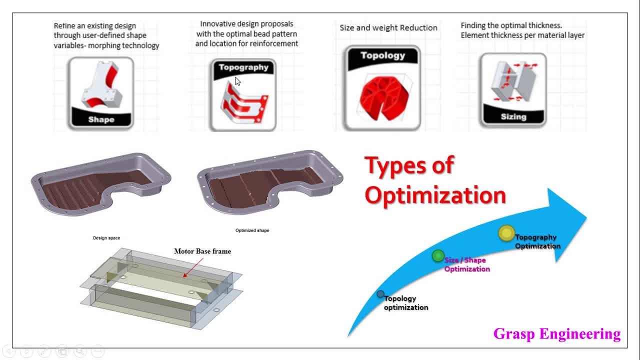 what your shape optimization. the next is your topography optimization. so here like innovative design proposals with the optimal bead patterns and location for reinforcement. so basically, it is used in order to create a reinforcement with the help of bead pattern. so let's talk about this example here. it is a simple bracket and this is what our design space. so now you will find that 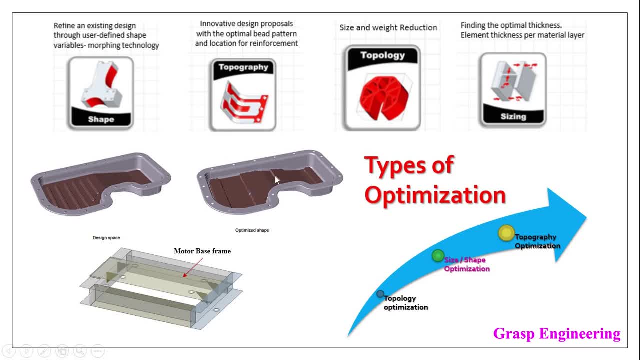 it will be optimized shape with the help of such a bead pattern. so that can be done with the help of topography optimization. and next is nothing but your topology optimization, as we discussed earlier. so here we can easily reduce the size as well as weight, as well as mass. so that is comes under the topology optimization. and the fourth one is like: 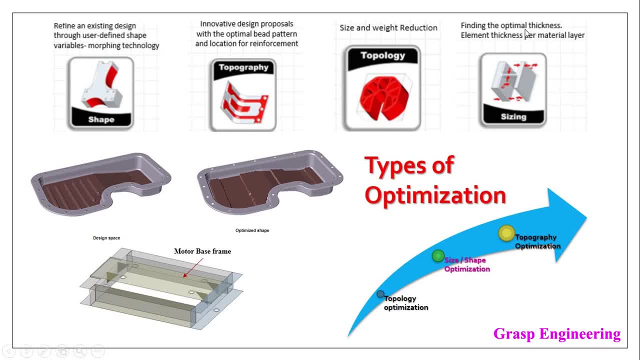 sizing optimization. so you are finding the optimal, like minimum thicknesses as well as elemental thicknesses per material layer. so here, with respect to elemental layer, we can easily identify the thicknesses. so when we have a shell type of structure, let's talk about this motor base frame. 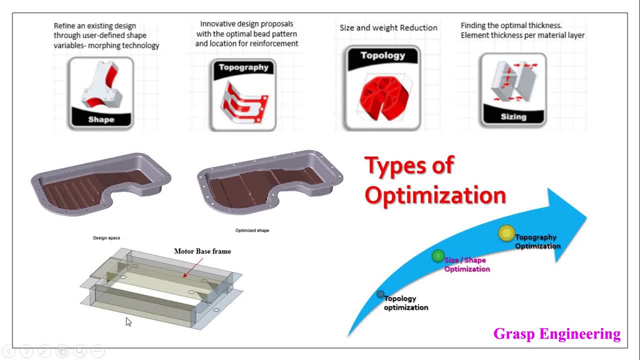 here you have a shell structure, so here when we are using sizing optimization, so in that case we can easily find out the minimum elemental layer thickness and it will also depict the various thicknesses, so on which thickness we need to consider, so that can be easily identified with. 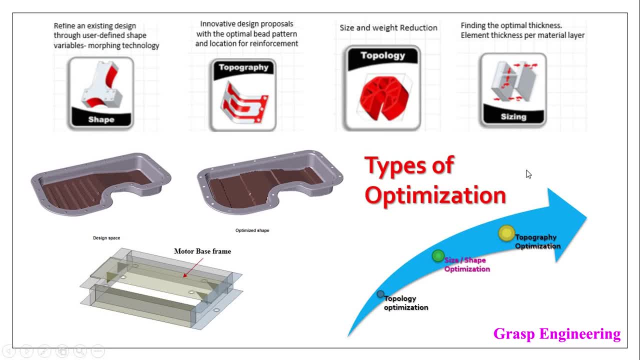 this help of sizing optimization. so all this optimization technique you will find in other simulations, optimization software, like when we talk about hyper mesh, Opti struct. so Opti struct is one of the best software which are used for a topology optimization. but nowadays ANSYS also came into picture and they also started giving competition to this other softwares. but 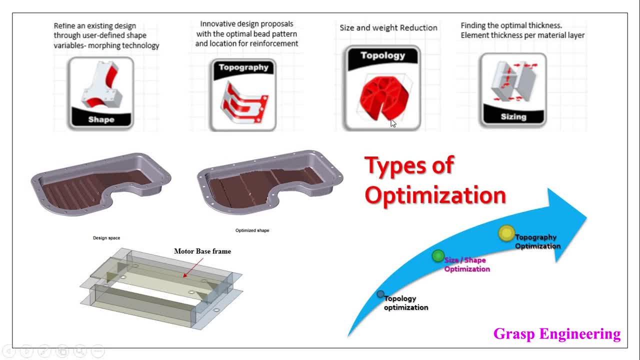 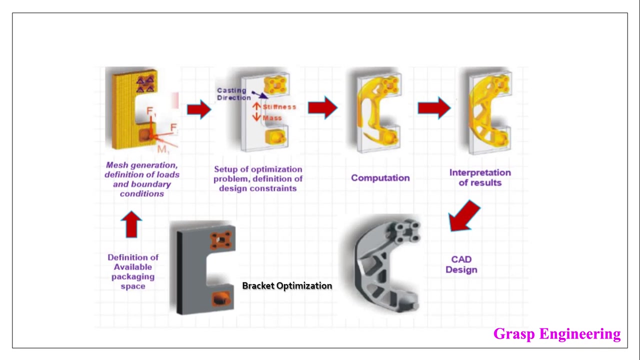 ANSYS nowadays offering only topology optimization. still they will. there are no offering for topography or other sizing optimization, so with the help of ANSYS, you can easily work on this topology optimization. discuss a few example and what are the major parameters which we needed. so this: 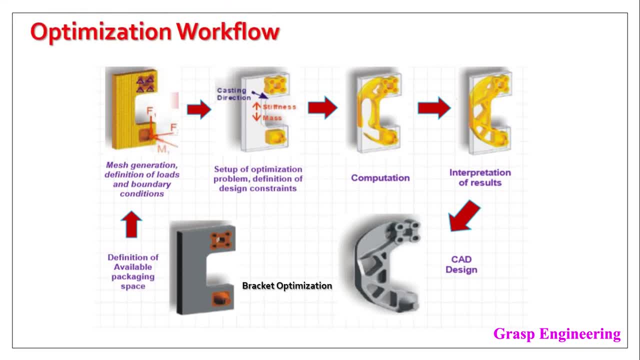 slide represent the optimization workflow. so when we talk about optimization workflow, so at the start we have a simpler geometry. you can see, this is what the simplified bracket, so it is what you can, a definition for available packaging space. so you have a bracket and you have a design space, like here: 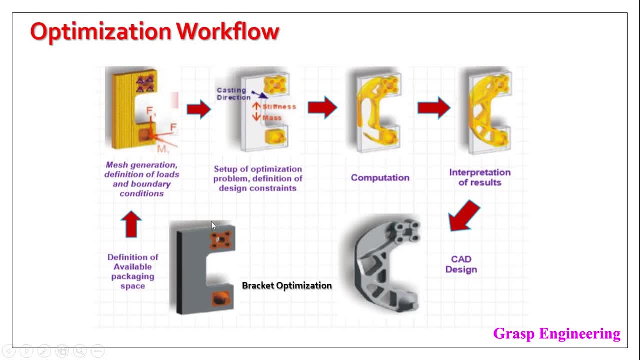 you need to define the constraints. now you can see here, here I want to define a constraint and here there is a load. so based on this to design space parameters and based on these loading, you put this into your simulation software and there you can generate the mesh, you can define the respective loads, you can apply the. 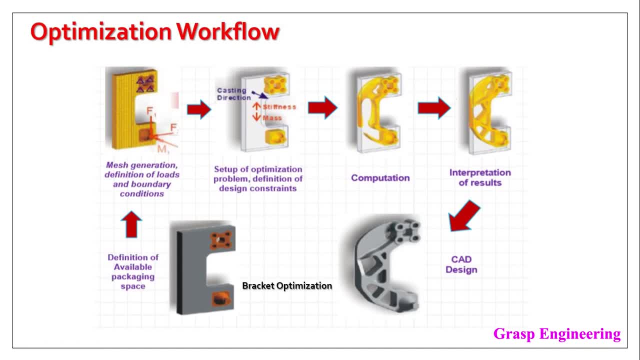 boundary condition. so all this can be done in your optimization software. once you have setup is done, then set up for optimization problem: definition of design constraints. so basically, you can define the design constraint. you can define the objective, like reduction in mass that we will discuss in next slide. 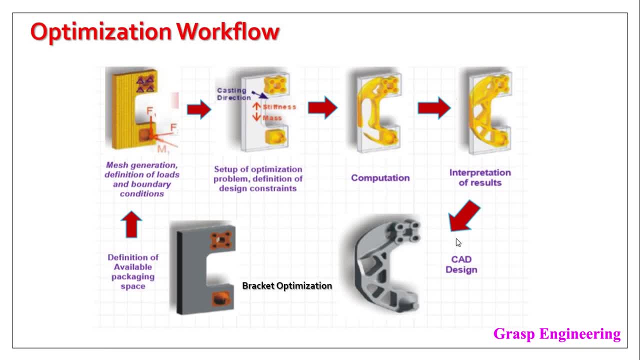 in more detail. what are the constraint on what of the objectives? so once you have defined objectives, once you have defined constraint in your optimization tool, then you can easily calculate the optimized shape with the help of your optimization software. so once our calculations are done, after the, you know your iterations are that- then you can. 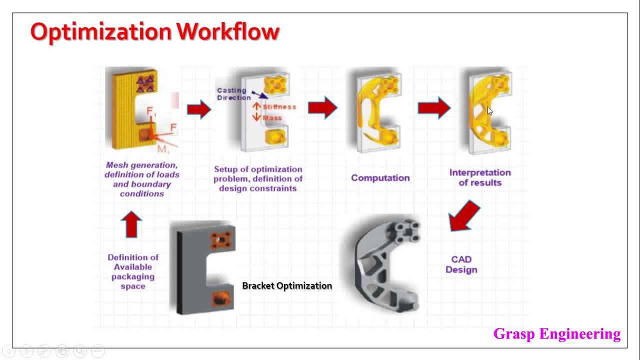 find out the final shape like this: so once you obtain the final shape from the initial shape, then you can interpret the results and then you can finally do the CAD designing, or you can finally define the CAD model for that respective optimized shape. so later on, once your CAD design is done, then you will find the 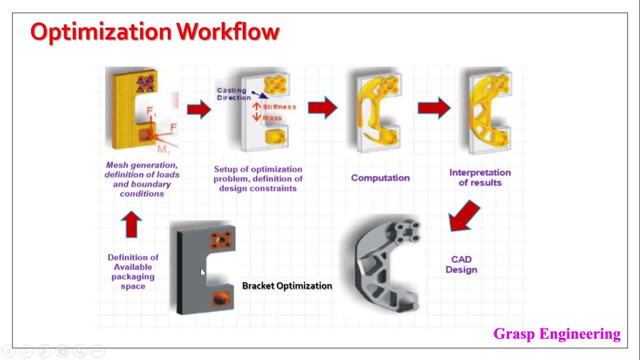 shape like this. so from this initial shape of a simple rectangular to that, after defining various parameter, of the defining various optimizations, like you can see the bead patterns here you can see the sizing optimizations. so, like that, you can play with this various optimization tool and later on you 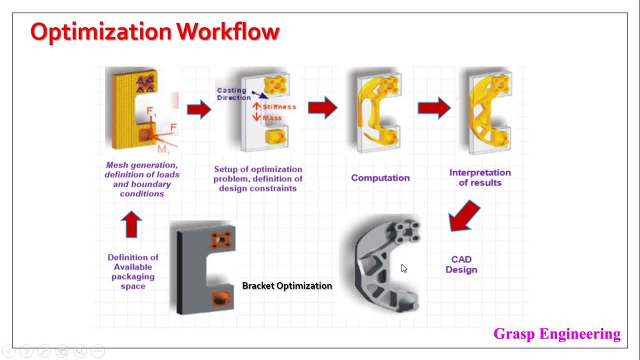 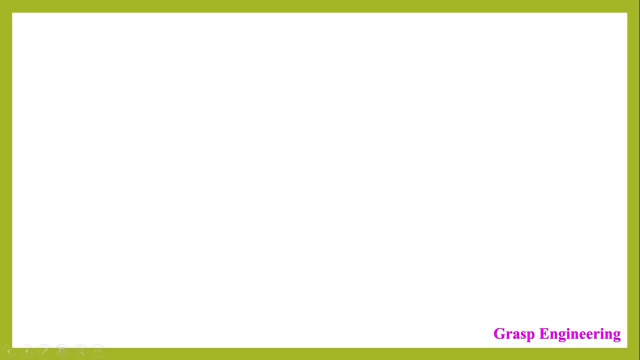 will find the optimum shape, like that. so which will be useful, which would have a more steepness and which will be useful further, the respect to reliable purposes. so like that you need to work and like that you will find the optimization softwares. now, this slide represents the physics and objectives. so now let's talk. 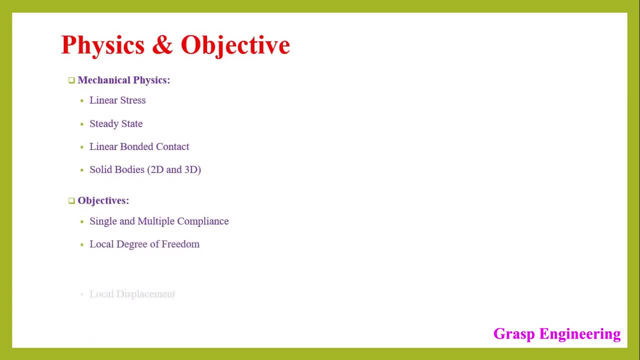 about the actual ANSYS topology optimization tools and what it's offering. so when we talk about mechanical physics, it offers four physics like linear stress, steady stress, linear bounded contact, solid bodies, 2d and 3d. okay, so for this respective physics we can do the topology. 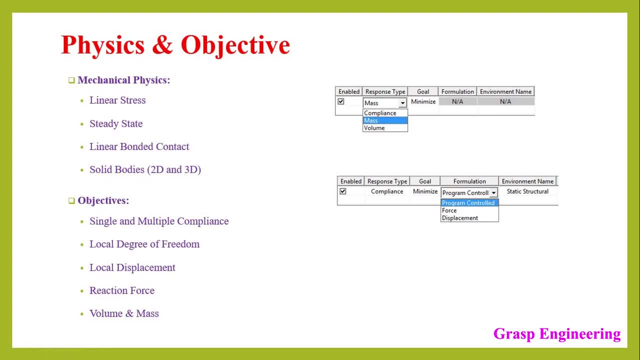 optimizations and then next talk about the very important thing, that is, objective response. so when we talk about, talk about topology optimization, so in that case we should have some objective why we are doing that so like, are we doing for a volume reduction in volume, are we doing for reduction mass? so all 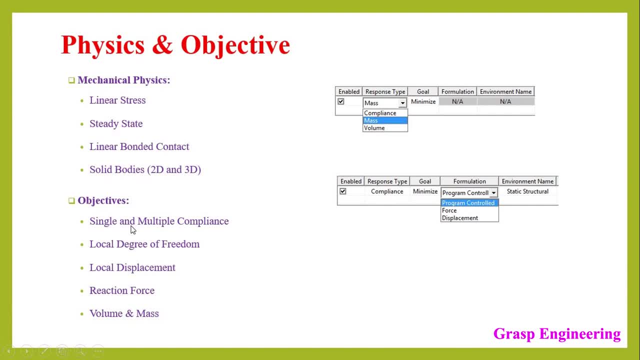 this you can see like we can do objective response, like single and multiple compromise. we can different find local degrees of freedom, local displacement, reaction forces, volume and mass. so with this parameter we can define the objectives. suppose you want to reduce the mass for the structure, like 50% mass. so you can define if you 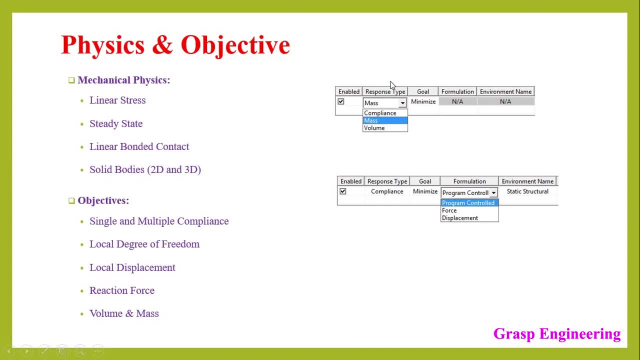 want to reduce the volume, then you can define with the help of response time, and even you can play with this force and displacement. so these are the major objectives. so when we talk about topology optimizations, as we know that we should, either we want to reduce the volume or we want to reduce the mass. so these are the two. 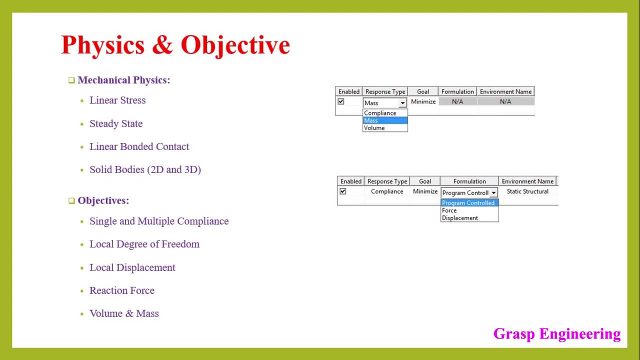 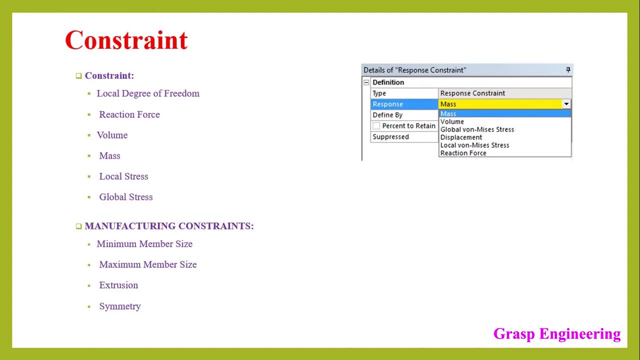 major objectives for any optimization simulations. so thus we can define in answers, mechanical, the next terms, very important terms comes, that is constraints. so when we talk about constraints so there are, like we can define local degree of freedom, we can define reaction forces, volume, mass, local stress and 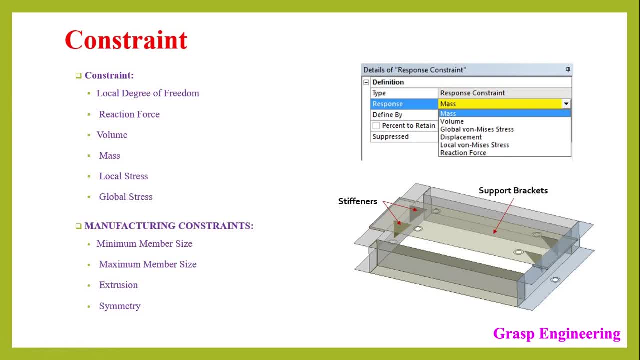 global stress. so for all these respective response constraints we can perform the simulations. so what exactly it is like, suppose, when we talk about global stress? so either you can keep the yield stress or you can keep the ultimate stress. suppose you have kept it a steel. for a steel, yield stress is like 250 mega. 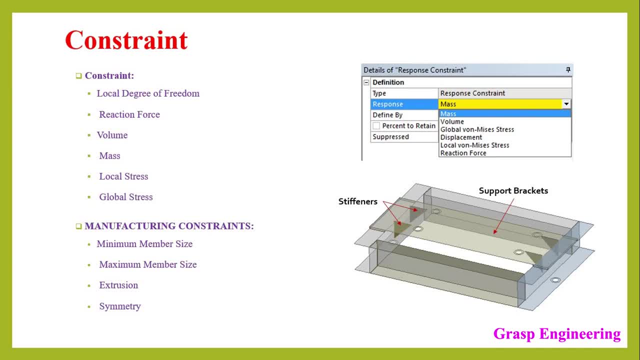 Pascal. so I want to define a global stress like 250 mega Pascal as a constraint, so that, based on this parameter, this topology optimization simulation will be performed. so, like that, you can define a volume, mass reaction forces, local degrees of freedom as a constant. the next very important term: 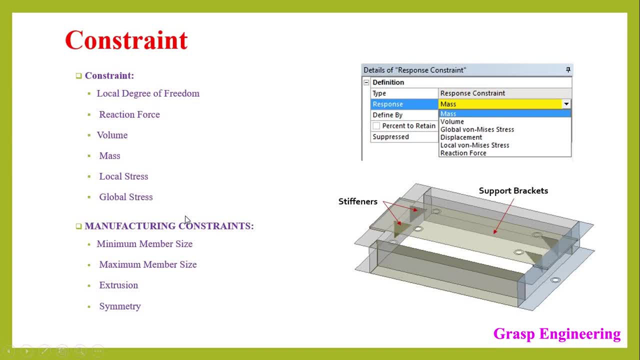 like manufacturing constraints and in addition to that, we can even define the manufacturing constraints like minimum member size, maximum number, size, extrusion are Symmetr, so you can. when we talk about response frame, so you just need to select these constant strains out of this force. and when we talk about 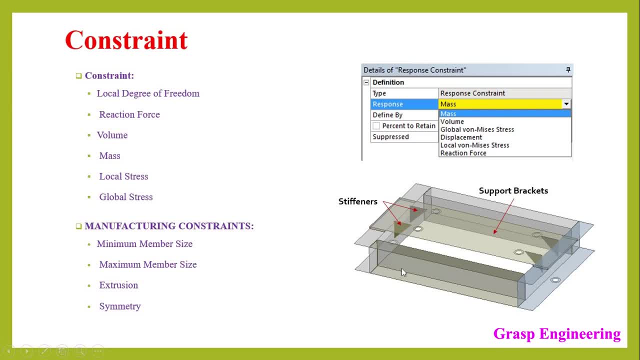 manufacturing constraints, suppose. take example of base Milano. so here we know these minimum member size for this supporting brackets, as well as size for this strip. now, so that can be defined with this help of manufacturing constraints. okay, now let's talk about one of the practical example of topology. 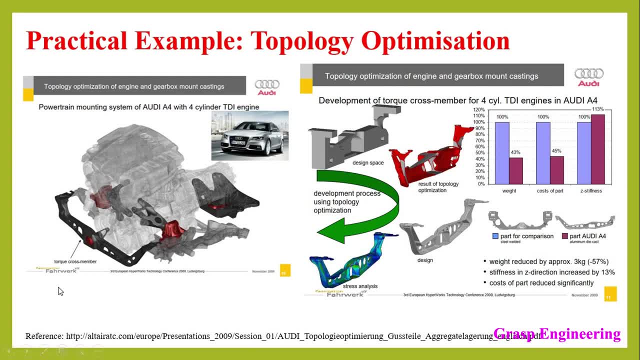 optimizations. so you will find this torque cross member which they have designed based on their optimization studied, and you will find the reference somewhere here at the bottom of this. so what they did here? so this torque cross member is basically a powertrain mounting system of Audi A4 with 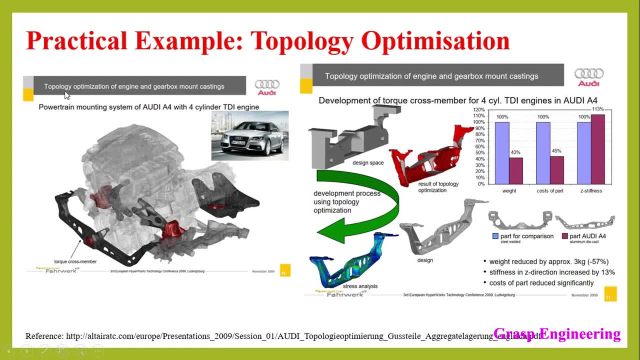 four-cylinder TDI engine. so it's nothing but your topology optimization of engine and gearbox mount casting. so here initially they created a design space like that, based on their respective parameters, so you can easily define something like this and you can easily define something like this, and you can easily 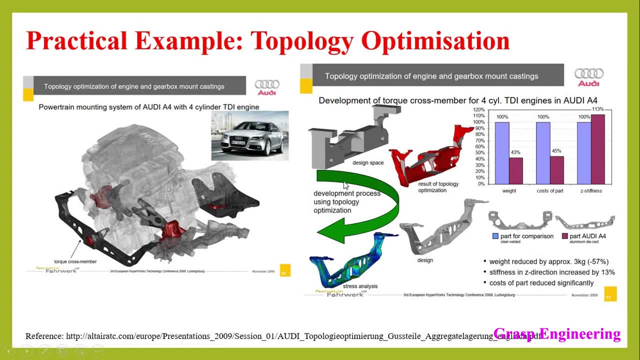 the design space. once your design space is defined, then you can put that into development process with the help of topology optimizations. and once you had defined various optimization processes, then you will find the results of topology optimization. like that and then further on, after being fine-tuning you. 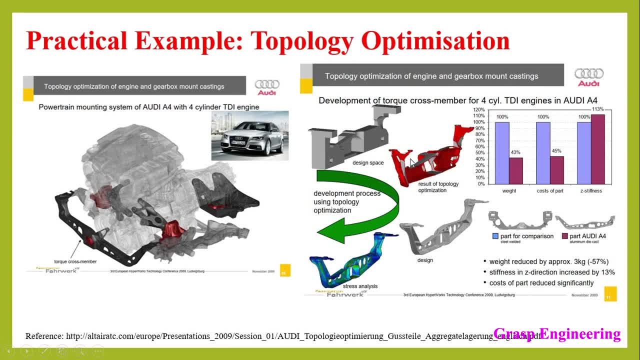 will find a design like this and once design is obtained with the help of optimization, then you can do further: a validation analysis, trace analysis, so you can find out the similar process and you can find out the design process, what we discussed earlier. so like that, from design space to a final shape. so 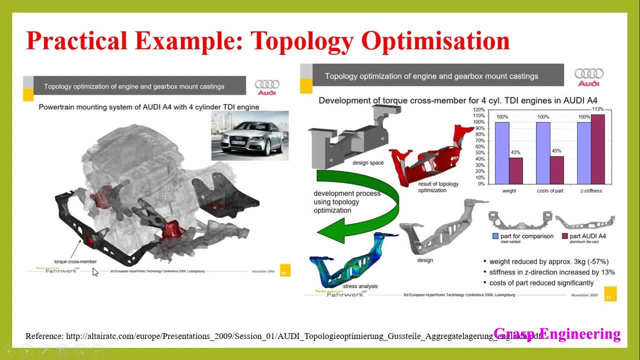 basically they did for their respective torque cross member. and what are the beneficial or what are the advances they obtained? like you see here, they got the weight reduction by 57 percentage, that is, approximately 3 kg, and the steepness in Z direction increased by 13%. cost of the parts reduced. 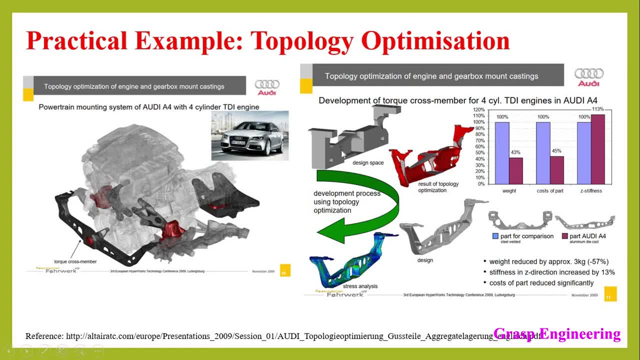 significantly. so what are the objectives they defined? based on that, they find out these outcomes. okay, so basically, here you will find initial hundred percent and then reduction of 57 percent weight. at the same time, cost is also reduced and at the same times their shade direction steepness is also increased. okay, so that is what the wonder, or that? 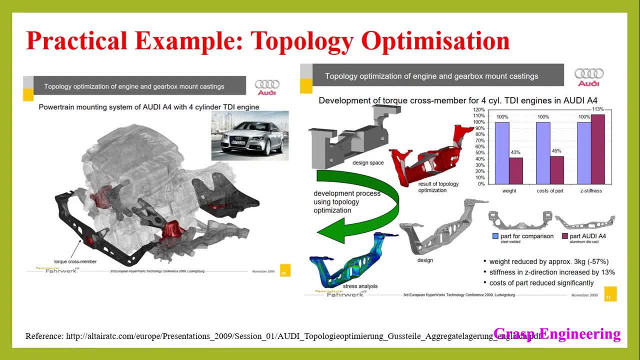 is what the advantage of doing optimization studies? you will also find so many other examples for this optimization. you can go through that. okay, then what we can do, we can go to our answers and there I will show you a simple study: how the workflow in answers, when we talk about answers mechanical- how it works, okay, so. 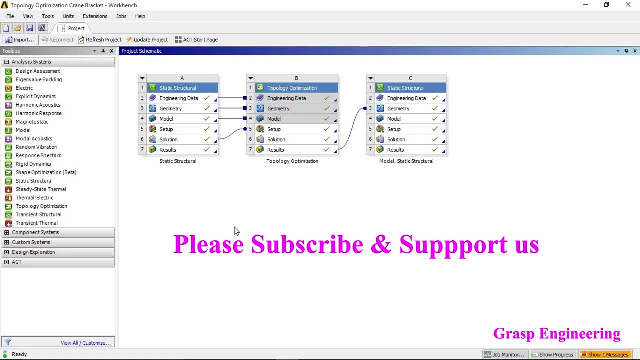 now we are, in our answers, mechanical. so here, very first you need to perform the static structural simulation and then you can connect that with its. this static structural simulation you can perform with respect to your loads and boundary conditions and then you can carry that results to your topology of the. 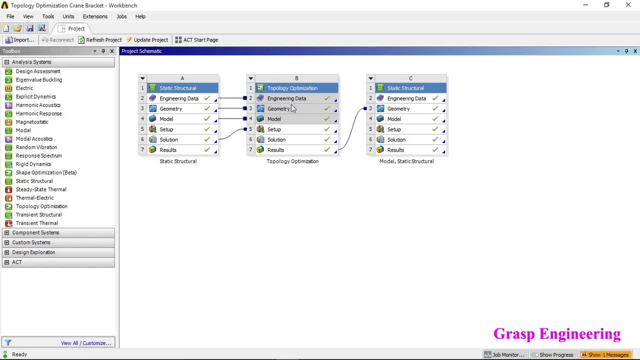 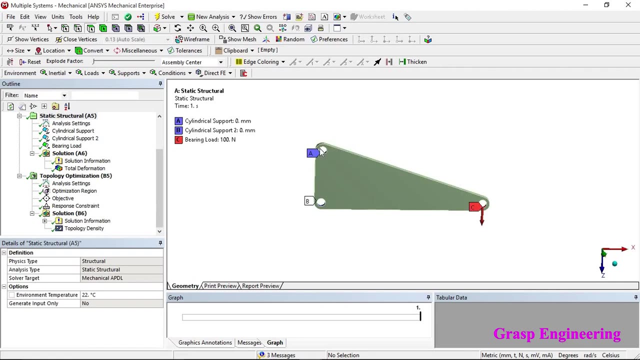 object and where you can define your constraints and objectives. once your constraints and objectives are defined, then you can further do the validation for your respective object. let's talk about one of the example of simple bracket. so here you can find out, here we have defined the constraints and here we 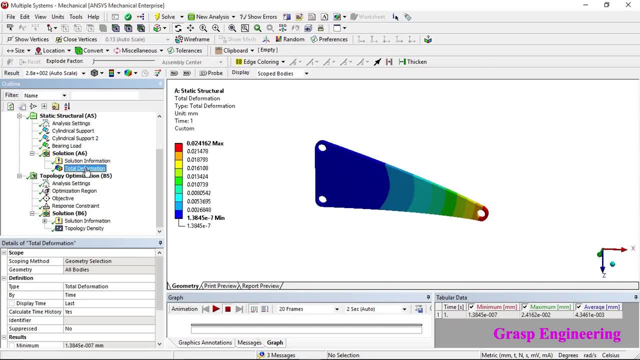 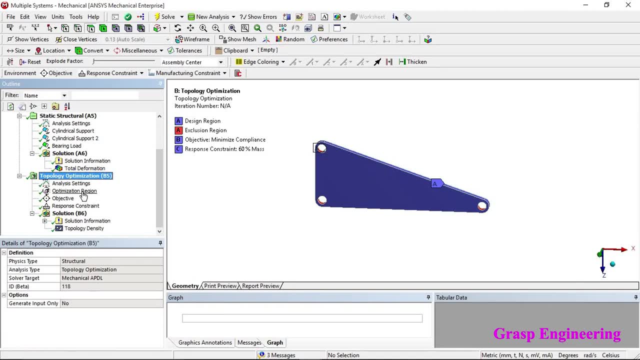 apply in the bearing load for that respect to you will find the deformations. okay, now you can find the deformation, and then these results are carried further and here we define the optimization reason. so you can see here: design reason indicated by this blue color and excluded reason is basically the constraint, as well as loading. 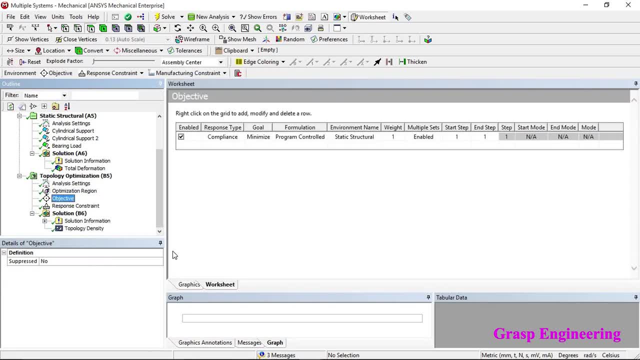 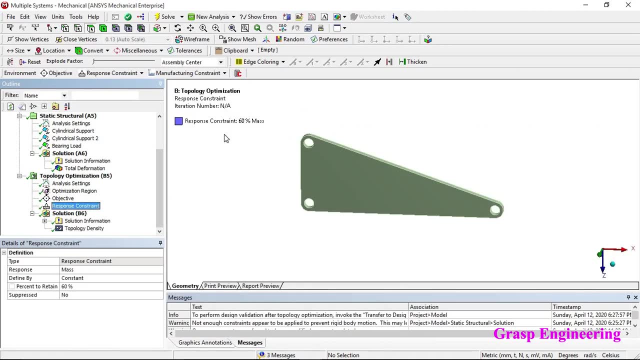 phases. and then here you will find the one of the objective, as, like, you can need to define the minimize, the masses, and here you can define the constant, like 60% mass. so what we discussed earlier, like, here you can define the constraints, the objective as well as constraint objectives that we need to.